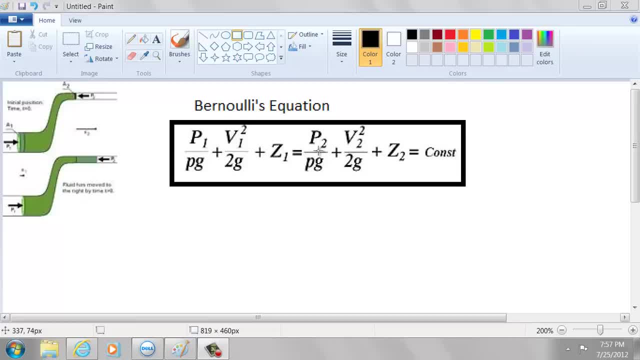 P1 is equal to P sub 2 over rho g plus v squared sub 2 over 2g plus z sub 2 is equal to some constant. We see here in this diagram, we have some fluid flowing. When you apply pressure to it, fluid of course is going to move to the right more. But what also happens is that while this pressure, becomes greater, this pressure also becomes greater. Even though the fluid is moving, it's not because there's less pressure, there's more pressure over here. But the pressure is becoming just as great on the other end to help slow down and equal this type of pressure on the other side of the tube. 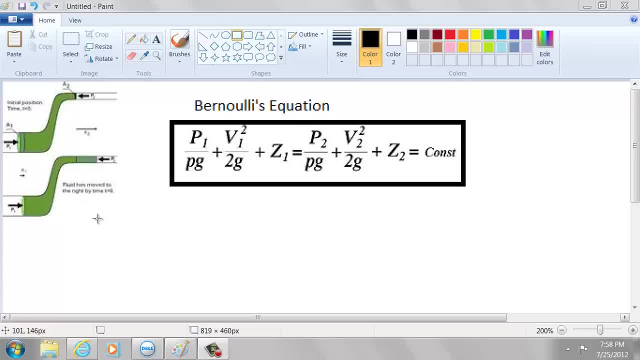 And that's what Bernoulli's equation is stating. Now there's a working form of Bernoulli's equation that's important. For this chapter. 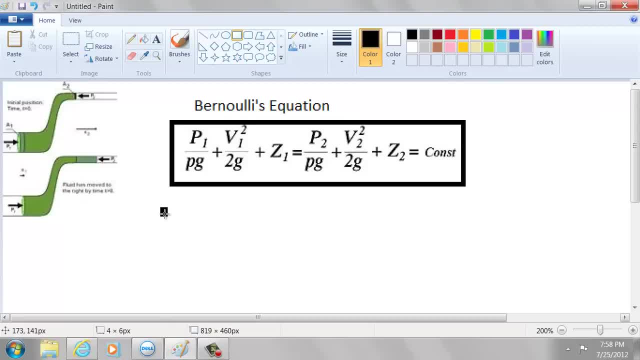 I will write it out for you. That was not correct. I will write it out for you. I will write it out for you. I will write it out for you. 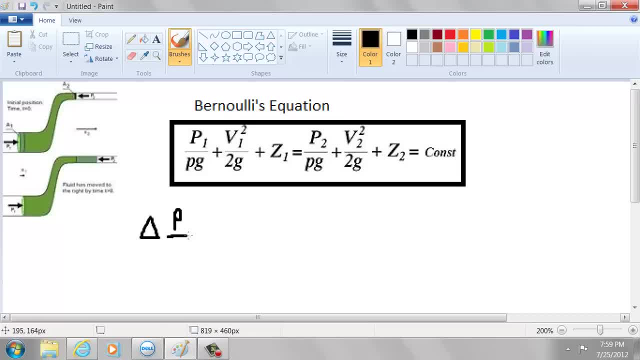 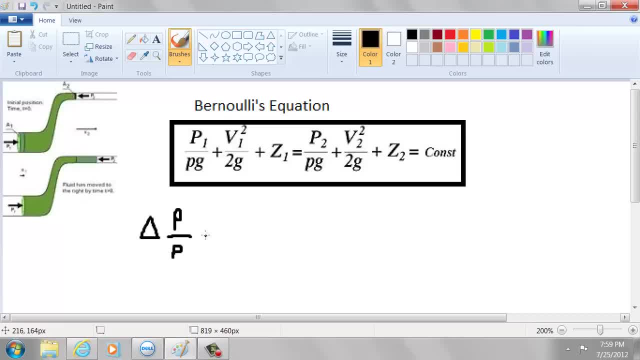 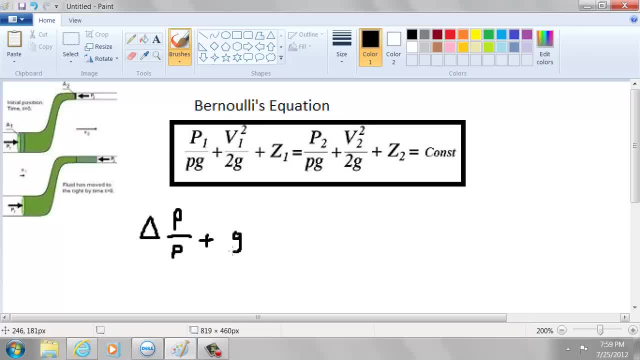 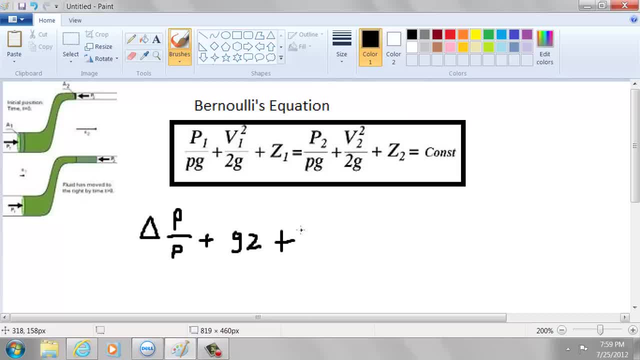 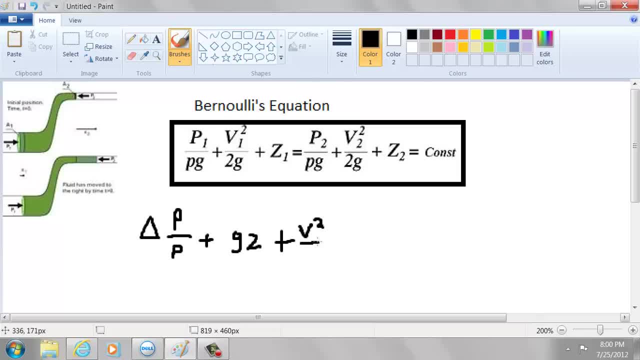 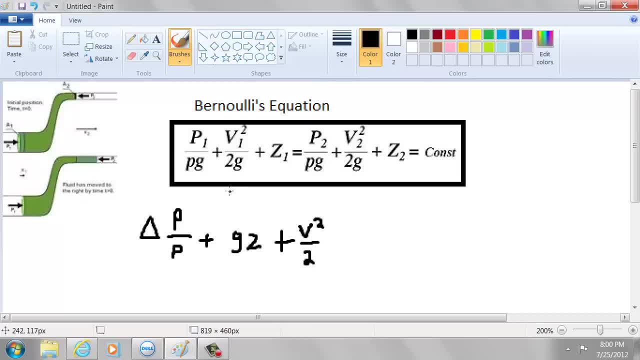 Thank you. Thank you. 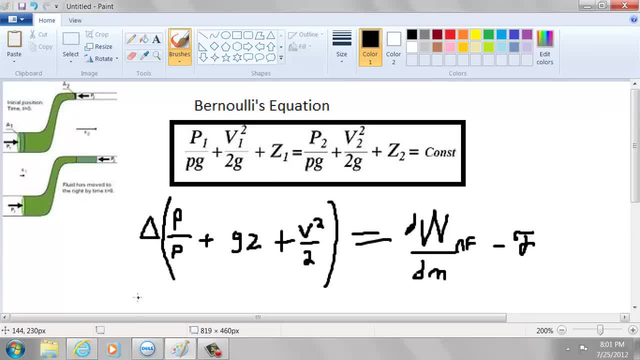 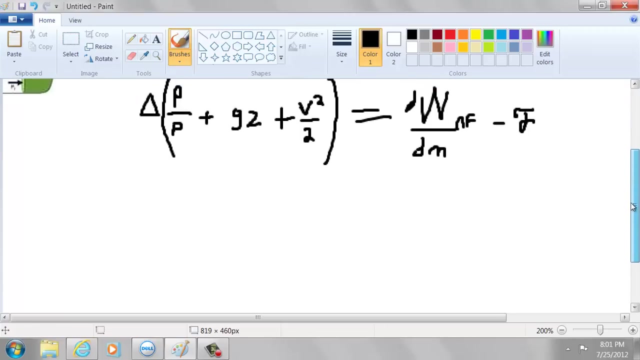 So this is the change in the pressure over the density plus acceleration times the height plus volume squared over 2 is equal to the change in work, derivative of work, non-force, over the change in mass minus the friction, friction heat per pound mass. And this is applied to problems in which we could set the friction term, this term here, the friction term right here, equal to 0. 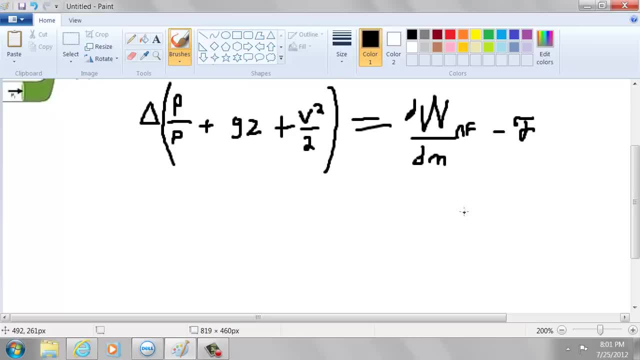 This chapter we show how to evaluate the term for the very important and practical case of steady flow in one dimension as in a pipe, duct, or channel. Using the friction terms we evaluate here. Sorry about that. 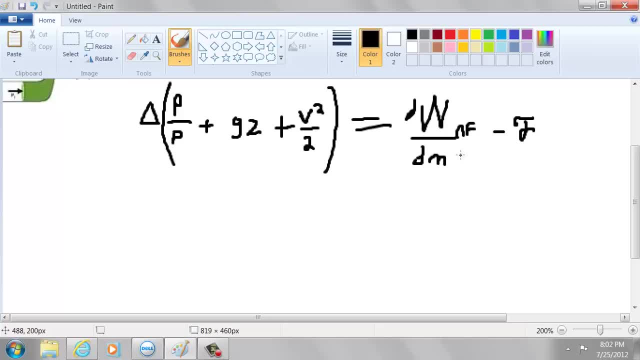 Using the friction terms evaluated here, we can use this equation for a much wider range of problems than those we have considered so far, including many problems of great practical interest to chemical engineers. 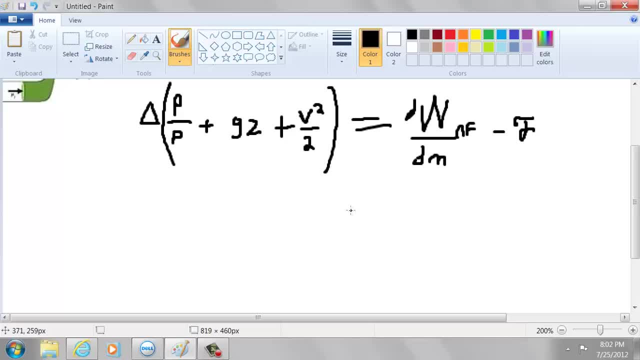 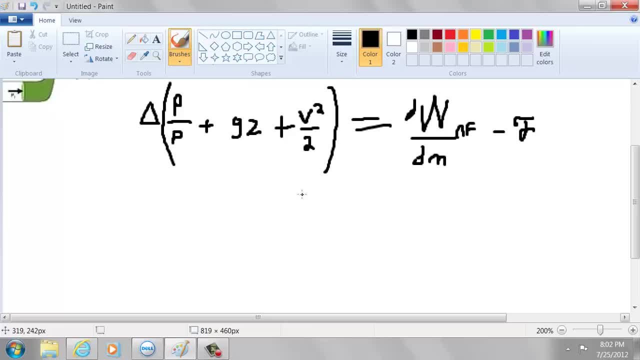 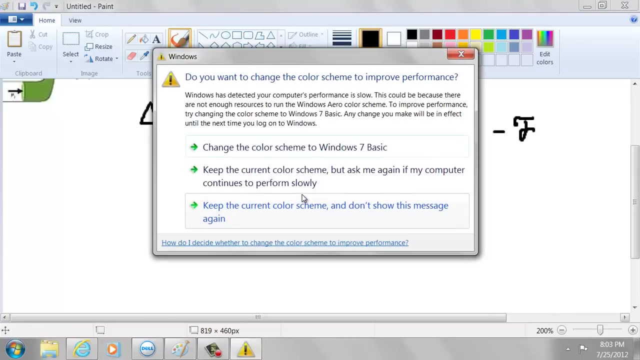 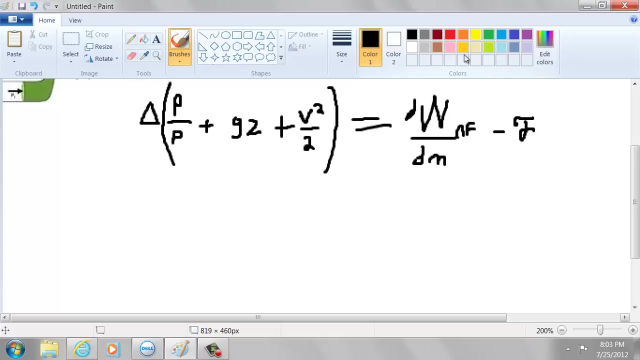 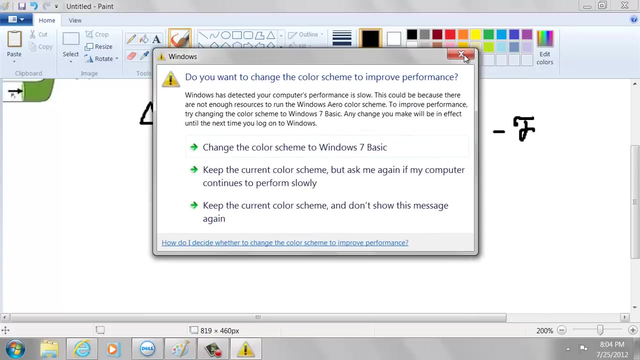 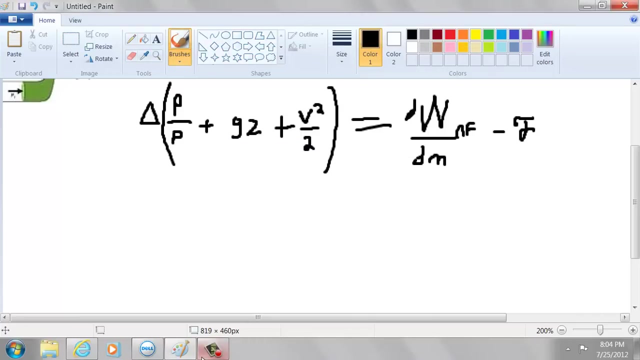 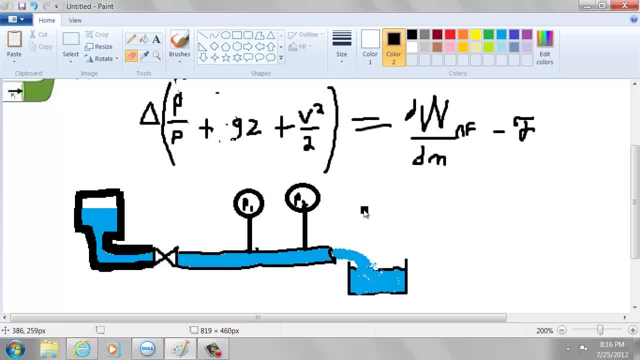 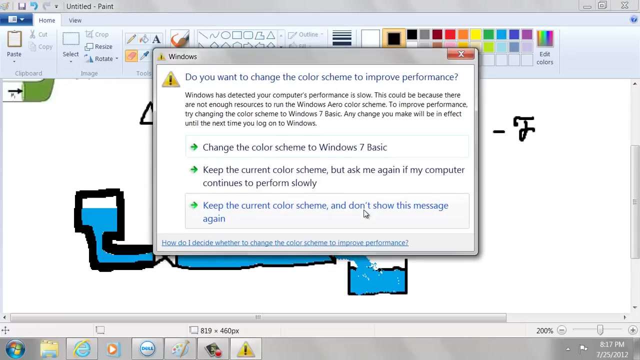 Regardless of what Newtonian liquid is flowing or what kind of pipe we use, the result is always of the form shown in figure 6.2. And for all gases at low velocities, the result is the same as that shown. Some features of one specific fluid flowing and one specific liquid flowing. Some features of one specific fluid flowing and one specific liquid flowing. 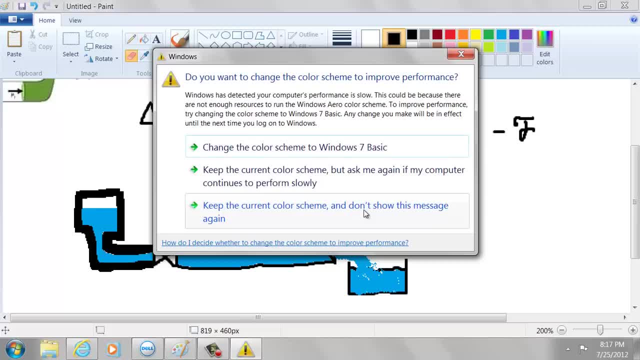 One specific pipe is that at low flow rates the pressure drop per unit length is proportional to the volumetric flow rate to the one power. At high flow rates, the pressure drop per unit length is proportional to the volumetric flow rate raised to a power that varies from 1.8 for a very smooth pipe to 1.3 for a very smooth pipe. 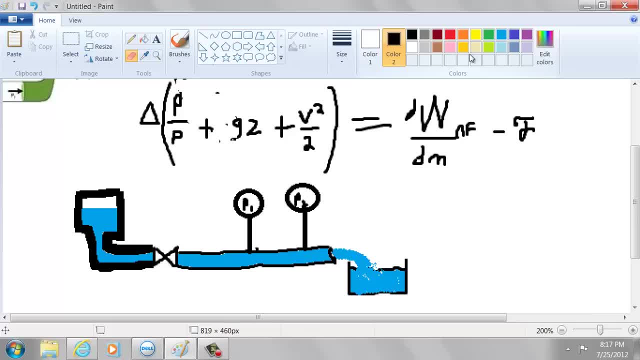 to 2.0 for very rough pipes. At intermediate flow rates, there is a region where the experimental results are not easily produced. The two curves for the other two regions are shown dotted extrapolated into this region. The flow can oscillate back and forth between these two curves and take up values between them. If the experimental apparatus is like that in 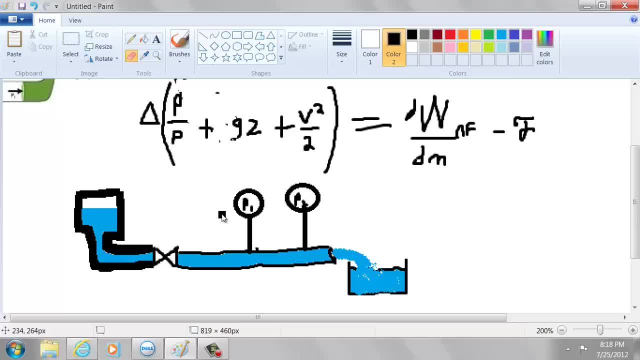 this figure, with a more or less constant value of dp over dx, pv in pressure, then the volumetric flow rate will oscillate horizontally between the two curves, producing an irregular pulsing flow. This is fairly blurry, but this is a graph of the flow rate. 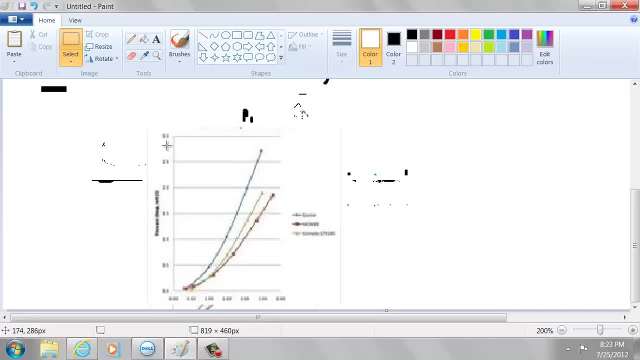 Pressure gradient, being on the y-axis, and on the left axis, the x-axis, is the volumetric flow. So we have pressure versus volumetric flow rate. And this is useful in pressure drop experiments. Down here, this is where negative dp is, and down here, this is where negative dp is. 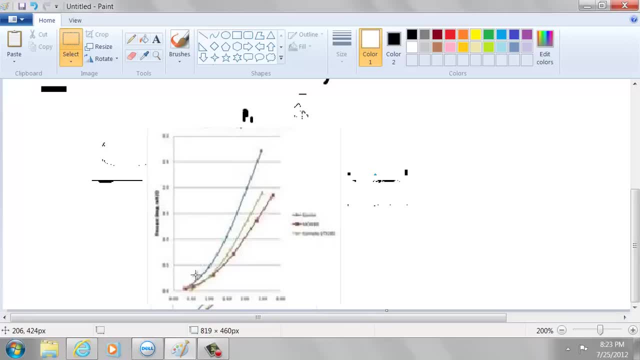 So this is where negative dp over dx is proportional to q to the 1 power. And there's sort of an unstable region where negative dp over dx oscillates between upper and lower curves. 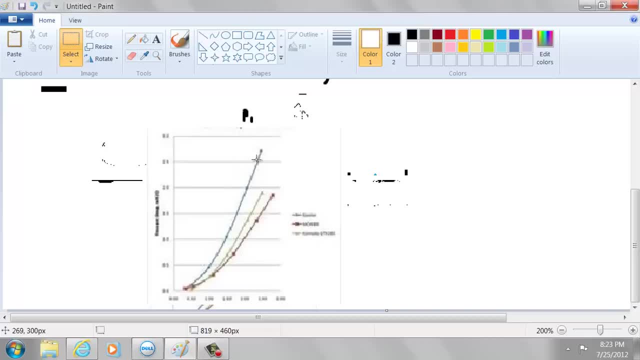 And then we have a region up here, where negative dp over dx is proportional to q to the 1 power. 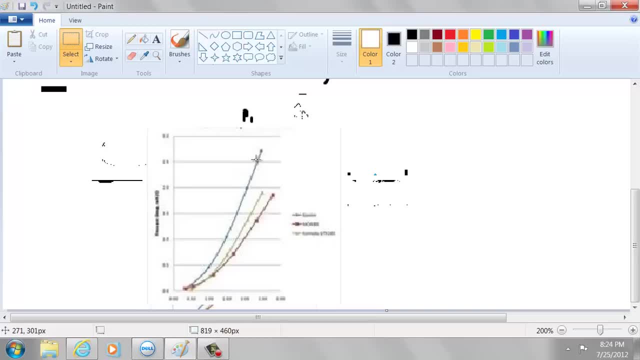 So we're on to the next question, where negative dp over dx oscillates between upper and lower curves. And we're going to draw something out here. 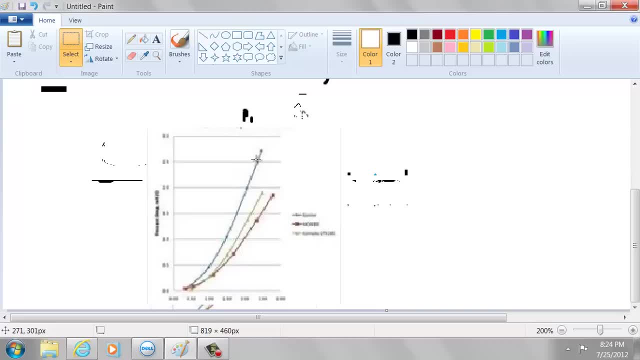 What does negative dp over dx say? 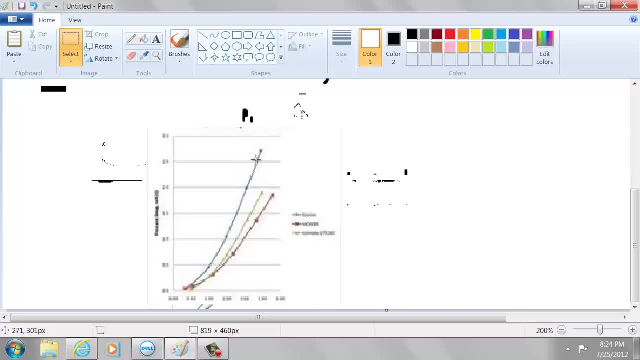 Well, now, the攻 peuvent être très rapides, mais très fortes. 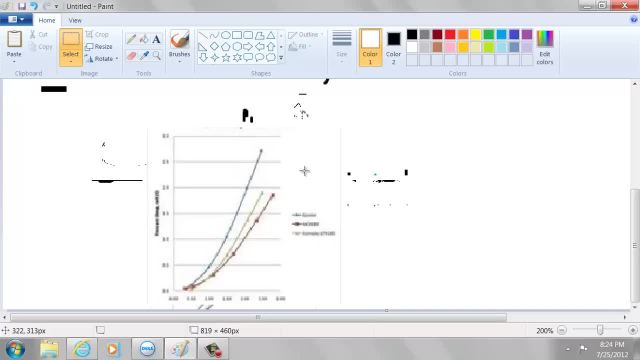 So the observer's going to go from a very fast pipe, which is very, very strong to the 1.8, or very rough, or very smooth pipe, rather, to 2.0, which is for a very smooth pipe, or a very rough pipe. 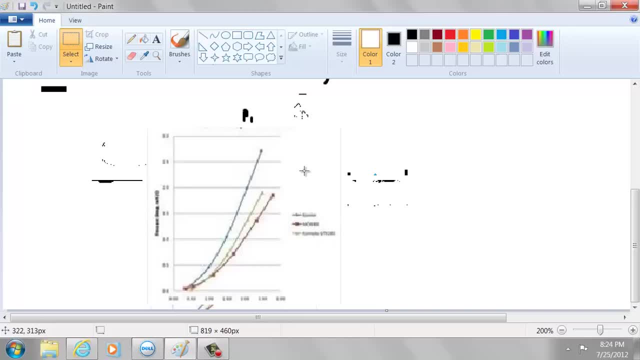 2.0 for a very rough pipe. Okay. Sorry, I kept on messing that up. But the main theory here, the main concept is that down here, negative dp over dx is proportional to q to 1 power. Here, it depends. It's between 1, it's between 1.8. It varies in between the two levels. And then in the high end, negative dp over dx is proportional to q to either 1.8, 1.9, or 2 power. 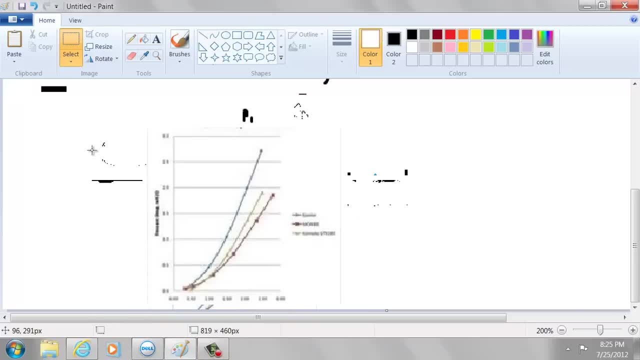 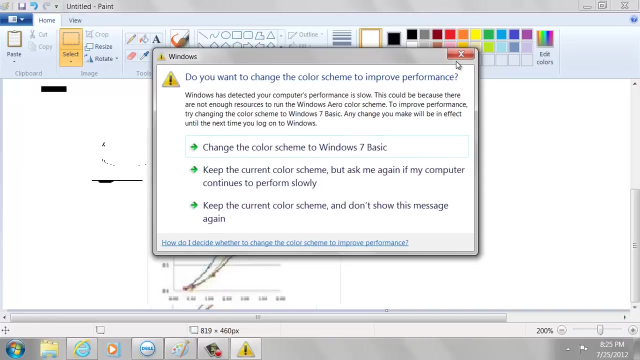 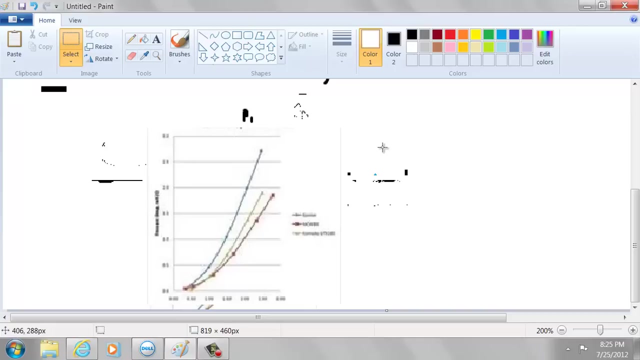 The experiment with the apparatus is relatively easy to run, and curves have been found for many combinations of pipes. However, since all possible combinations have not been tested, it would be convenient to have some way of calculating the results of a new combination without having to test it. Furthermore, no inquisitive mind will be satisfied with figure 6-2, this figure here, without asking why it has three regions so different from each other.